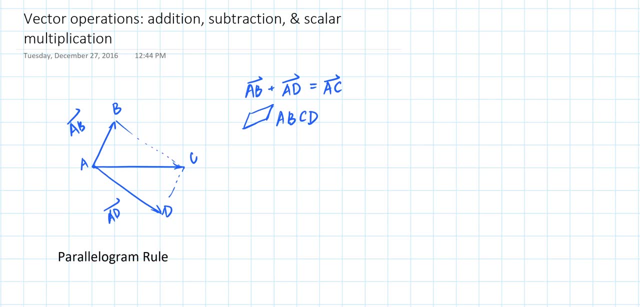 ABCD. you can notice that there are two pairs of equivalent vectors here. Vector AB is equivalent to vector DC because they have the same length and direction, and vector AD is equivalent to vector BC for the same reason. So if you replace the two vectors, you get the same length and 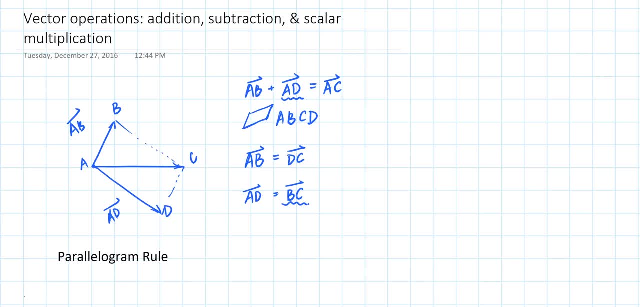 direction. So if you replace the two vectors you get the same length and direction. So if you replace vector AD with its equivalent vector BC in this equation, then this equation becomes: vector AB plus vector BC is equal to vector AC. This equation describes an alternative rule of adding two geometric vectors that's called 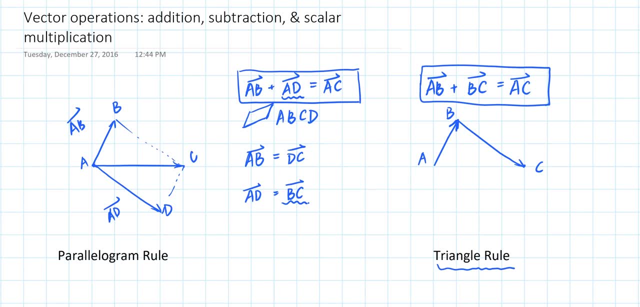 triangle rule. The triangle rule is useful when you have two vectors that are positioned so that the initial point of one vector is the terminal point of the other vector and in this case the sum of the two vectors is vector AC. You can remember it this way: 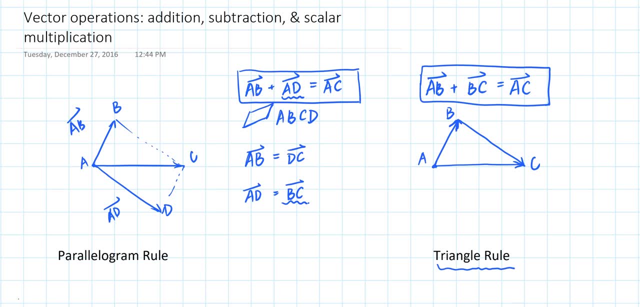 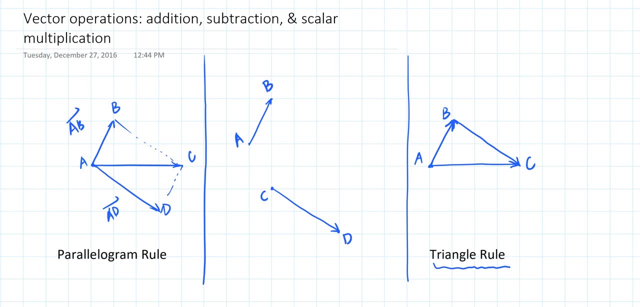 If you walked from point A to point B and then from point B to point C, then you effectively walked from point A to point C. Now what if you have two geometric vectors whose initial points and terminal points don't coincide at all? In this case, you can just find equivalent. 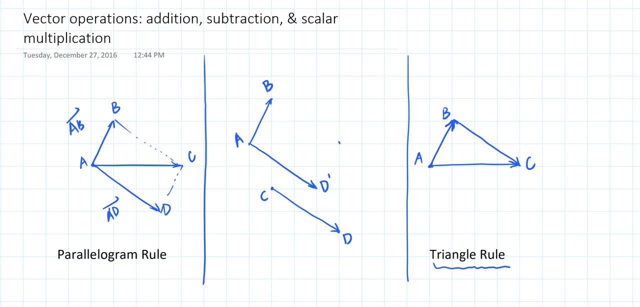 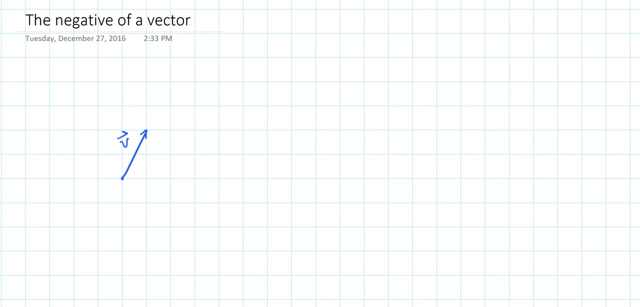 vectors of one of these vectors. so then you can apply the parallelogram rule or the triangle rule. Now let's move on to talk about subtracting two vectors. First of all, we need to learn about the negative of a vector. The negative of a vector v is the vector that has the same 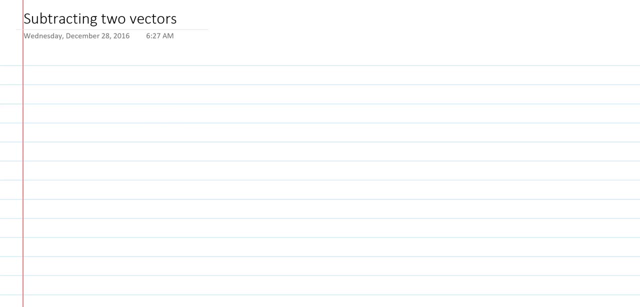 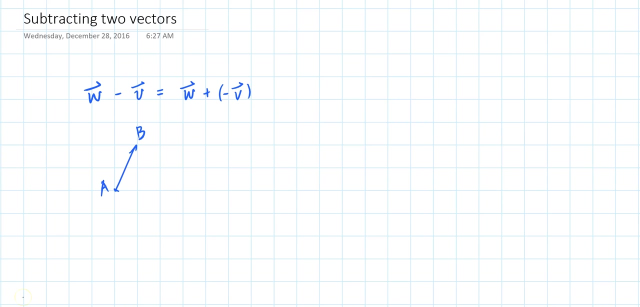 length, but the opposite direction of vector v. and the difference between two vectors, w and v, is the sum of the first vector and the negative of the second vector. so w minus v is equal to w plus negative v. So vector AB subtracted from vector AB is equal to negative. 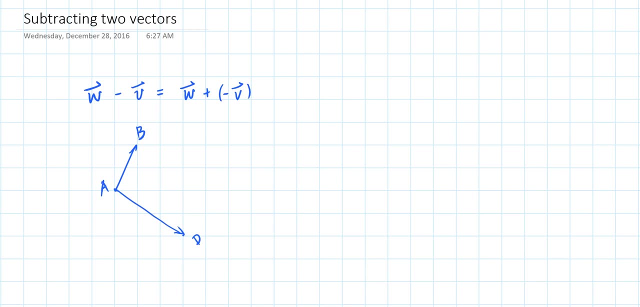 of vector AD. Applying the parallelogram rule, we find that AB minus AD is this vector AC. It is also true that the negative of vector AD is equivalent to vector DA. So, applying the triangle rule, we know vector DA plus vector AB is equal to negative of vector DA.